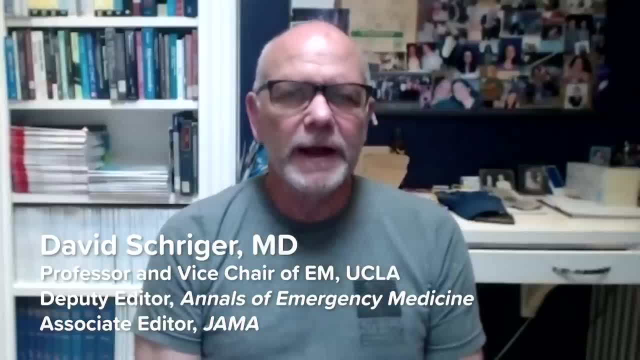 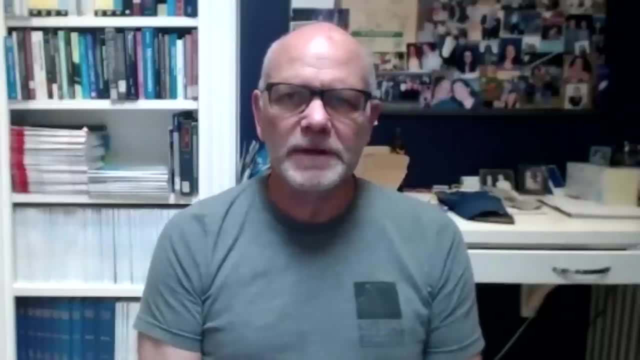 the last couple of weeks about the epidemiology of COVID And I wanted to continue today trying to figure out where we're going to go from here and also review to some extent some of the terms you've been hearing, like R0 and RT and herd immunity, just to give you another way of looking. 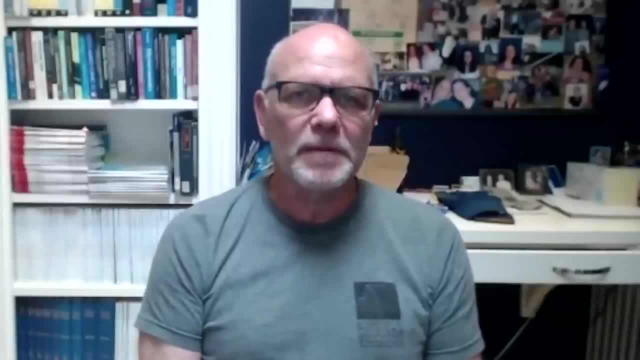 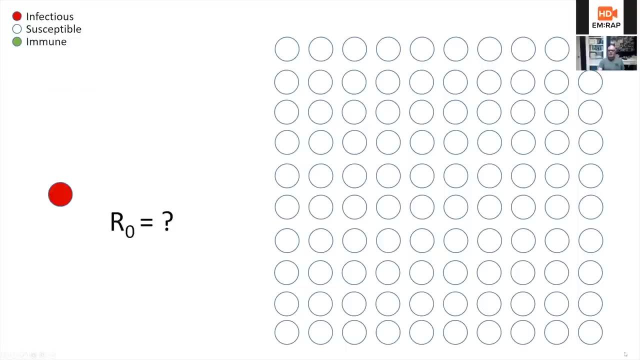 at these things. For many, this may be a review or obvious, but there may be a few of you out there who find this helpful, So we'll give it a go. So, first of all, this slide depicts 100 people who are vulnerable to getting COVID and one person who currently has it. What does this term R0 mean? 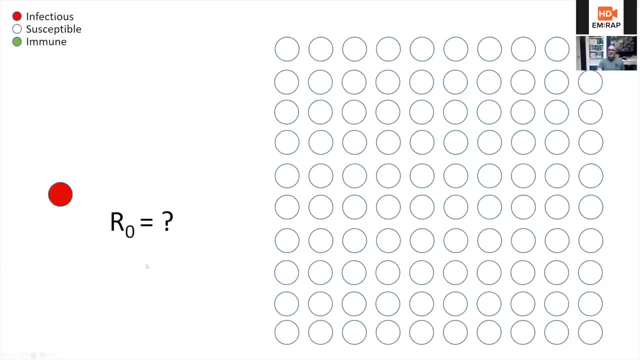 The term R0 is specific to a certain environment, a place and a time, even, and says: left to its own devices. how many people will get infected from this one person? So, of all these people that this person contacts, how many of them will get infected? That's all. R0 means Recognize that R0. 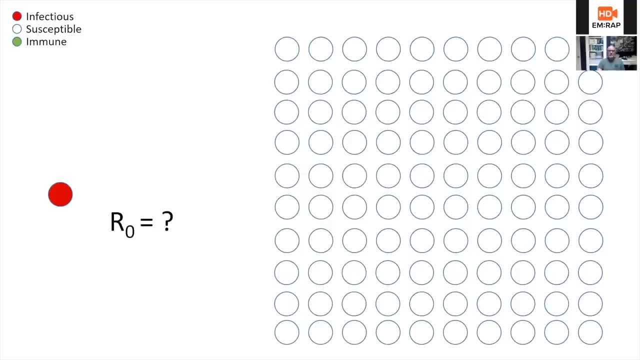 can differ from environment to environment, based on how densely populated an environment is and other environmental factors that we don't fully know about yet: Temperature, humidity, all kinds of other things. So that's what R0 means, And as an example, here's an R0 of 10.. Over the course of this person's disease, 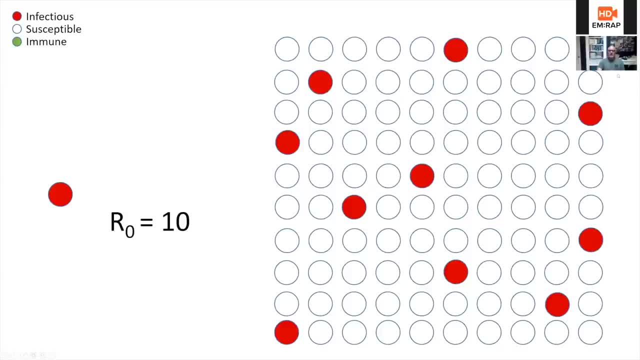 they're going to infect 10 people, represented by the 10 dots here. If that happens, the number of cases will increase linearly on a logarithmic scale, And this makes sense if you think about it. The first person that infects 10 people each of these infects. 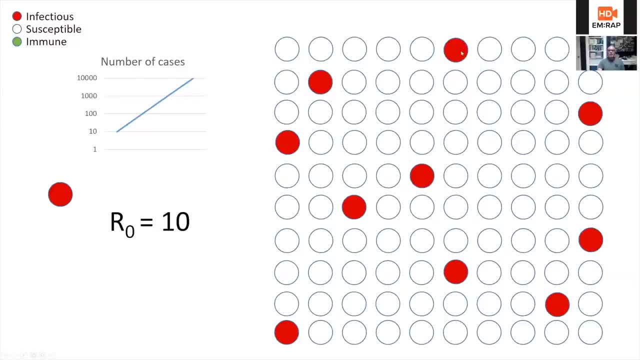 that's 10 times 10 is 100. Then those 100 people each infect 10 people, that's 1,000. And over this time period, whatever that transmission cycle is for this particular disease, we go up like that. If, however, we have an R0 of 2, this one person only infects 2 people. 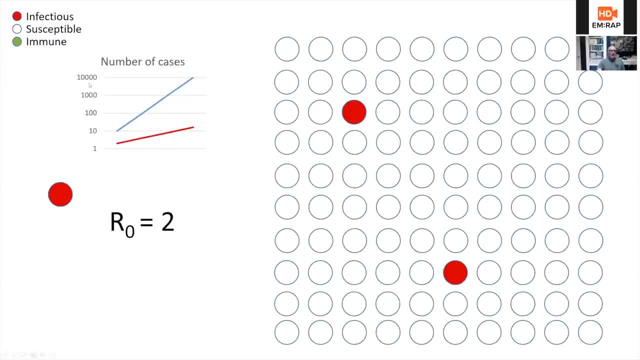 And consequently the slope again on a logarithmic curve is much lower. Finally, you can imagine that if R0 equals One, each person infects one person. I didn't draw the graph here, but you can imagine that there would always be a flat number of people. 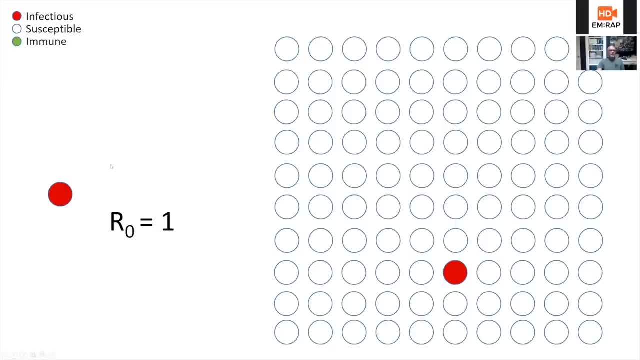 because as soon as this person has it, this person gets it. eventually this person doesn't have it anymore, this person still has it. So there's only one person who has it in the community and the disease would just kind of peter on. 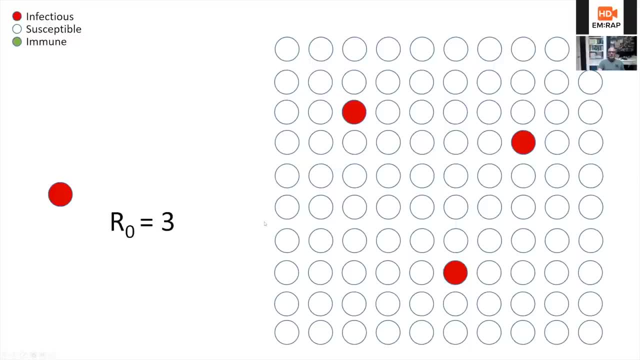 Three is a common number kicked around for this actual COVID infection, and that's what that would look like. But what we'd really like to know is not just R naught but what R T is. R T is what the actual transmission rate is. 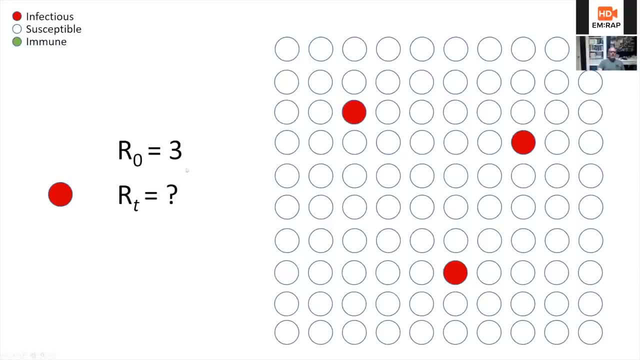 in the community at a certain time. And just because R naught is three, R T doesn't have to be three. For example, imagine we do something which is the opposite of social distancing. We make everyone go to political rallies every day. 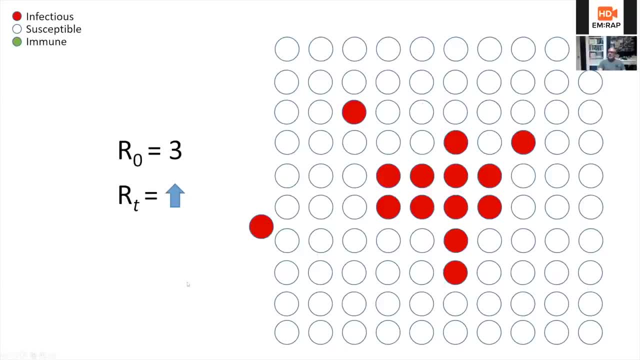 which brings this infected person in much more contact with all the other people and therefore, instead of infecting three people, this person infects this many people And obviously R T is much higher than R naught because in fact you've done social concentrating. 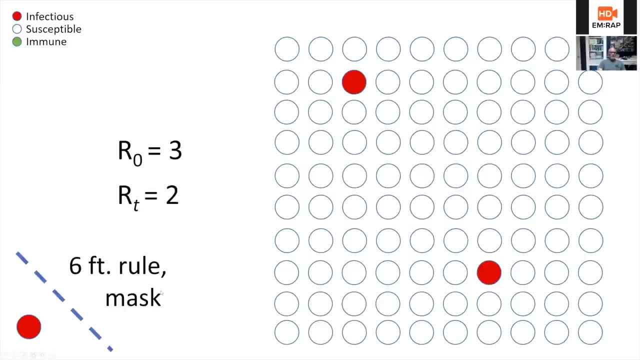 Alternatively, you could do things like a six-foot rule or a mask, which would decrease this person's transmission. And even though the R naught is three, in the presence of these things, R naught becomes two, Ideally for healthcare workers like ourselves. 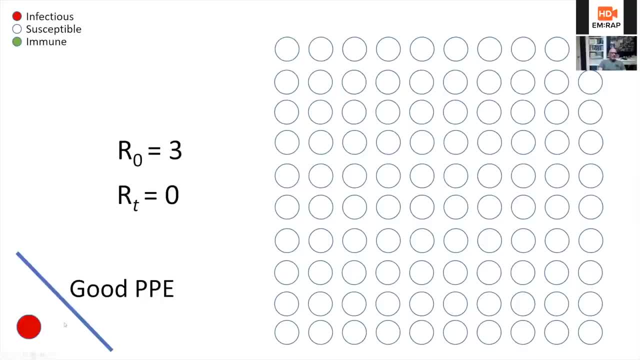 good PPE practices would set the standard, which would set the standard, which would set the standard and set up a barrier that gets R T to be zero even though R naught is three, and that no healthcare workers get infected, And clearly that is our goal. 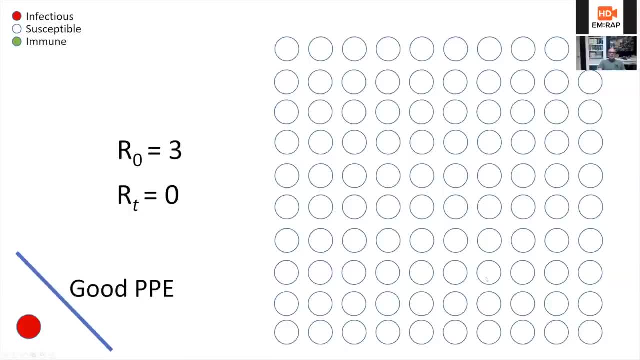 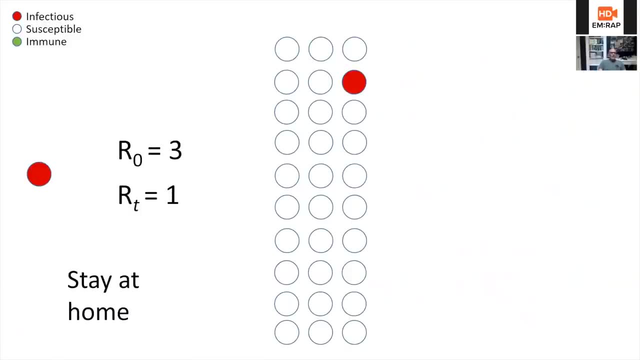 not currently an achievable one, but hopefully something we can move towards with better training, better availability of PPE and less of a surge condition. We try to stay at home. What does that effectively do? It decreases the number of people that this person is exposed to. 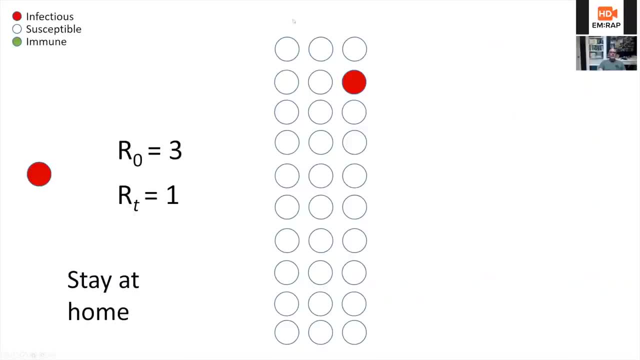 So instead of being exposed to, say, 100 people in their normal life, they're only exposed here to 30, and instead of three people out of that, 100 getting it, one gets it If we combine all these things, the six-foot rule. 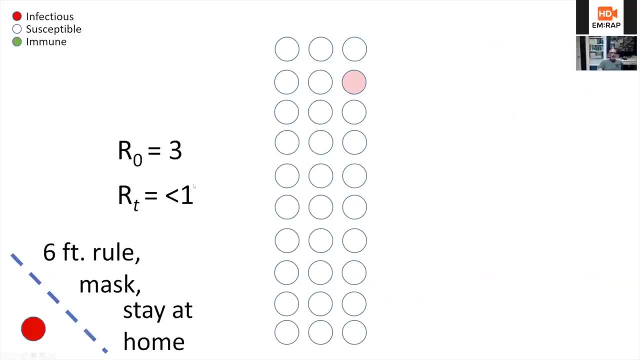 the mask, the stay at home. hopefully we could drive R T to less than one. When R T is less than one, each person is giving it. each person is giving it to less than one person on average and therefore, over time, the disease should disappear. 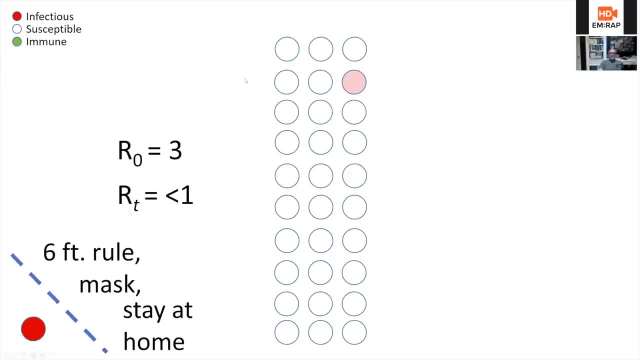 And depending on how much lower than it is in one, it dictates how long it takes for the disease to disappear. So all of these types of techniques can take a disease that has an inherent R naught of three and drive it below one. So if we want to get rid of this epidemic, 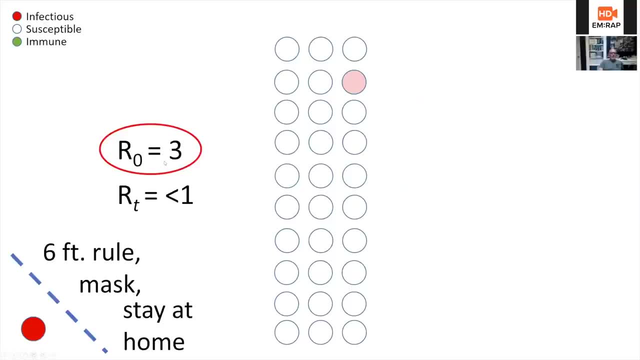 one way to do it is by techniques that decrease R T below R naught. The other possibility is that R naught actually might change. So imagine that miraculously, as some of the R naught approaches, as happens for many other diseases like the flu, R naught changes. 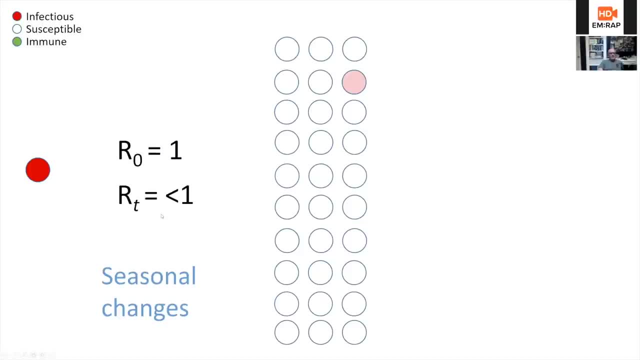 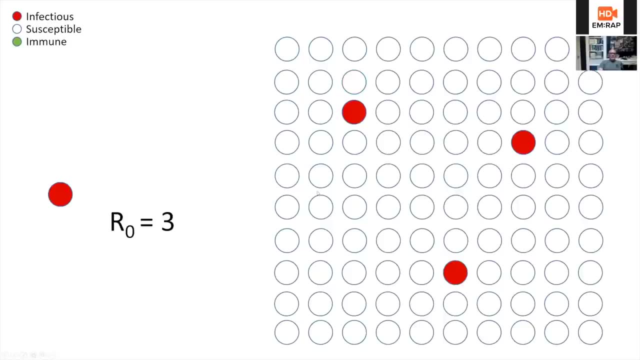 Well, obviously, R naught dropping down to one, with the other social distancing things in place would drop R T to less than one and we would see the disease decline in the population. But let's now start off with an R naught of three. 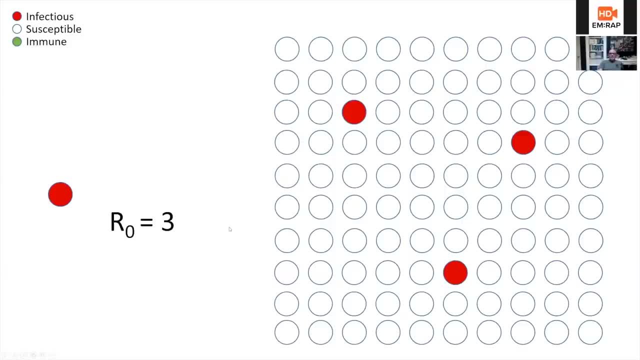 And let's assume now that we've been through this first cycle, The surge is over. The biology of the disease hasn't changed. R naught is still three. What happens next? Well, if miraculously, everybody already had the disease and everybody was immune, and that 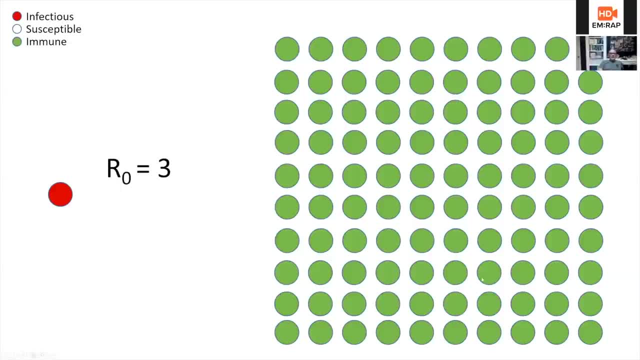 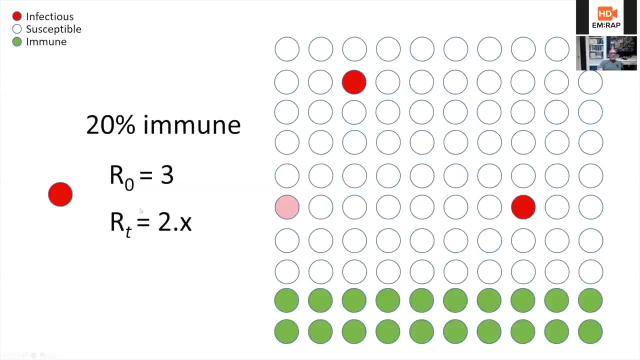 could be by everyone getting it or by a vaccine which we don't yet have. R naught could still be three, but R T would be zero in this case. If, on the other hand, we imagine that 20% are as immune, 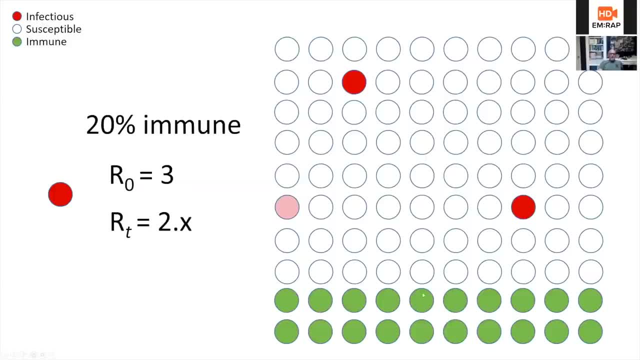 a number that's been kicked around as a high end estimate in New York. well, these 20 people are immune. That kind of takes them out of it. But even with an R naught of three you're going to still have, just by the mathematics of this. 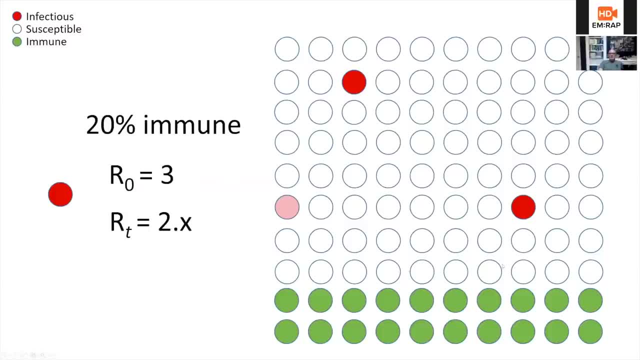 assuming that everyone who's susceptible is equally likely to get infected, you're still going to have an R T of 2.x and the disease will continue to grow in the community. And these numbers, of course, this is what forecasters spend their lives doing. 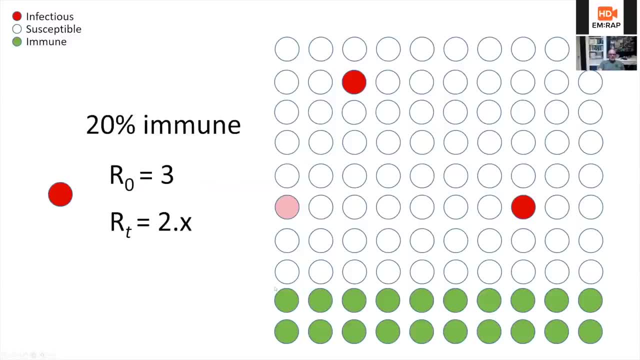 is trying to figure out what that x is For our purposes. just recognize that with this many people out, you still have transmission which is still going to be zero. You're going to have transmission which is above the magic number of one. 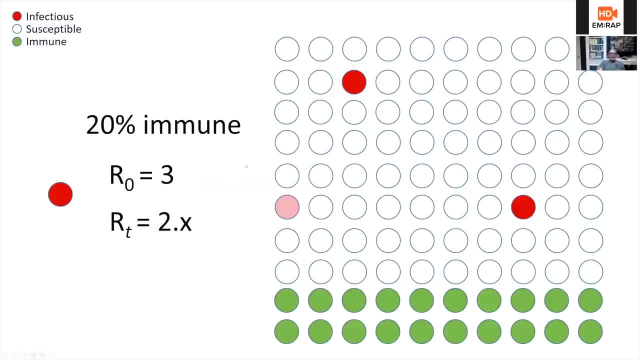 and the disease will continue to grow. And imagine that in places not like New York- most of the rest of the country- this isn't anywhere near 20%, It's more like a couple of percent, so that there are only five or six green dots. 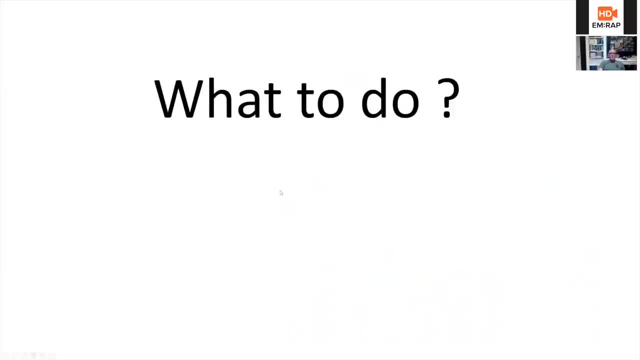 and the rest of these are all white. We're basically right back where we started from. So what do we do at this point? So what do we do? There are two main arguments that are in the mainstream media and out there. The first is: what do we do? 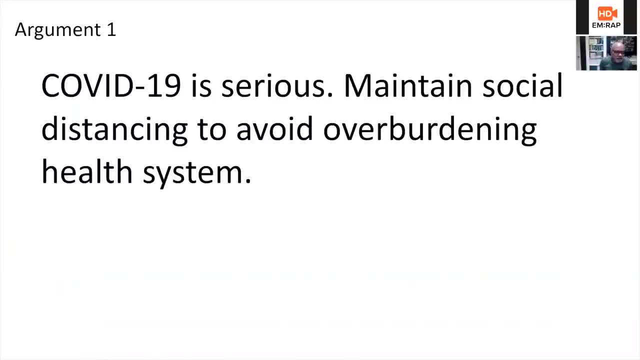 The second is COVID-19 is serious. We need to maintain social distancing to avoid overburdening the health care system and all the consequences of that, outcomes that are worse than they would be normally: health care workers who become ill, lack of health care workers, therefore, et cetera. 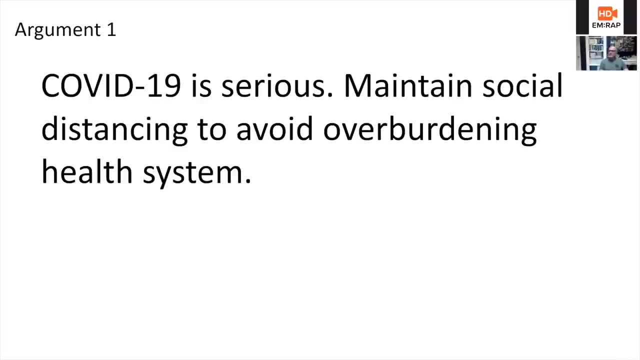 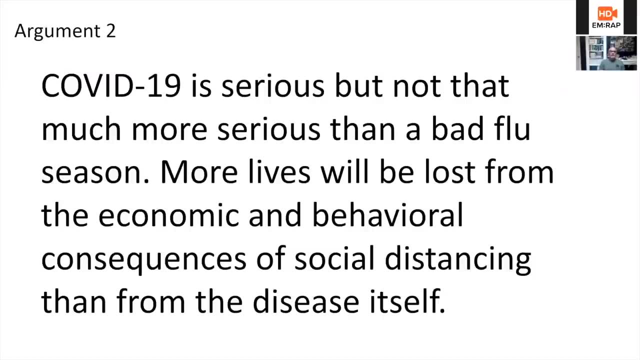 The other argument that's out and this argument. many people- Dr Fauci et cetera- have espoused this argument. The second argument, however, is that while COVID-19 is serious, it is not that much more serious. 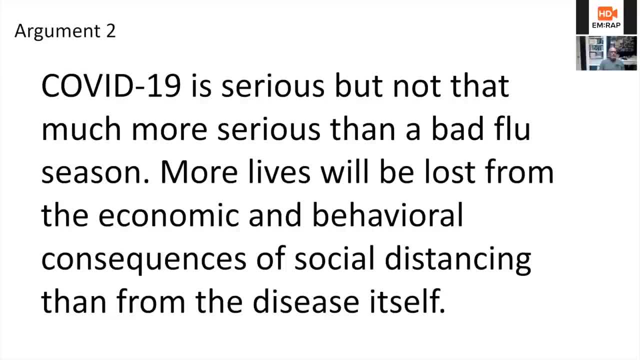 than a bad flu season. More lives will be lost from the economic and behavioral consequences of social distancing than from the disease itself. Now, of course, there are people who, under any number of different political theories, believe that social distancing represents a form of coercion. 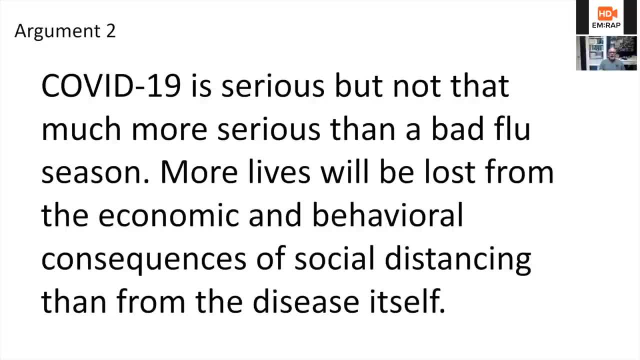 which is not appropriate for the government to do. But there are also legitimate academics and people who are very well thought of in the academic community who are making such an argument, such as John Yanidis. You can see his videos up on YouTube. 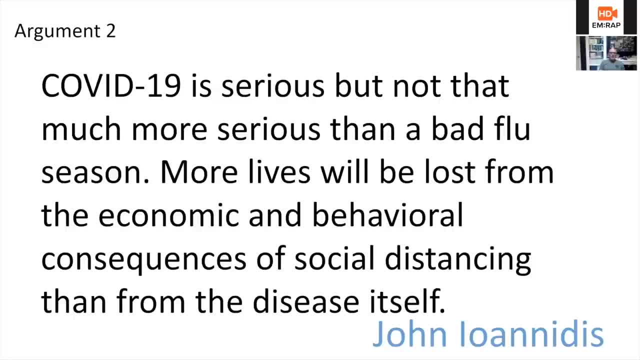 where he is interviewed for hours at a time explaining why he believes that the social distancing may be an overreaction to this problem. And unfortunately this whole argument one versus argument two has both been polemicized a bit as a political argument, with the left being with argument one. 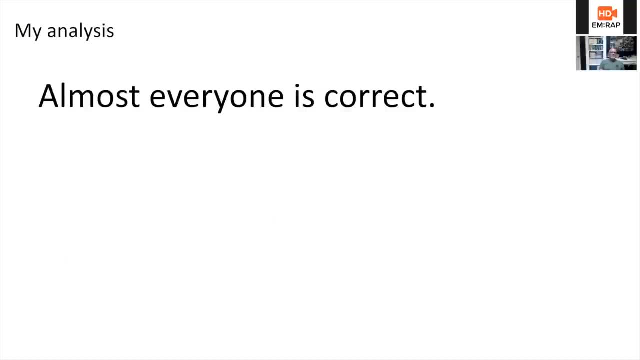 the right being with argument two- And I think that's unfortunate because I think almost almost everyone here can be correct, And let me explain why that is. I think what we're really seeing is the consequences in the United States of a highly managed, profit-driven health care. 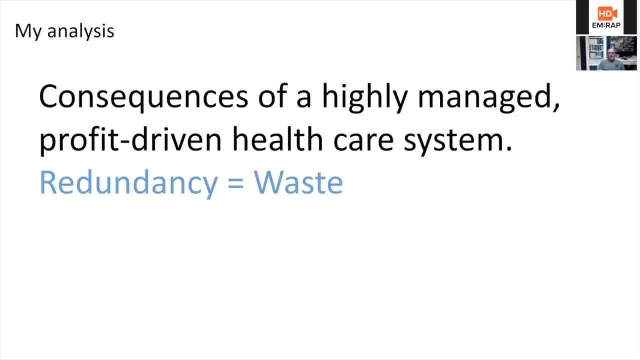 system. What do I mean by that? Well, first of all, in our current health care system in the United States, redundancy equals waste. If a manager sees a nurse who doesn't have many patients to take care of, or a physician who's 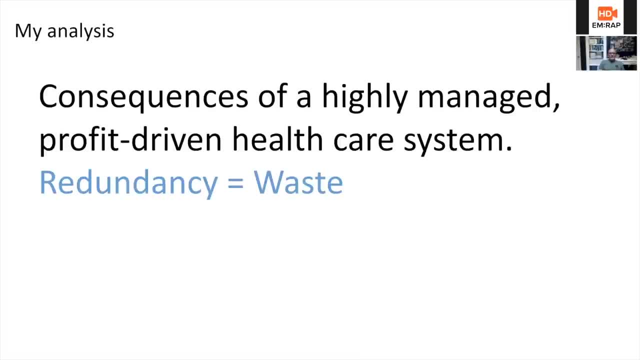 not constantly engaged seeing patients or beds that are not full. that's waste. Waste decreases profit and therefore it needs to be eliminated. But from a public health perspective one could look and say: redundancy does a number of really good things. 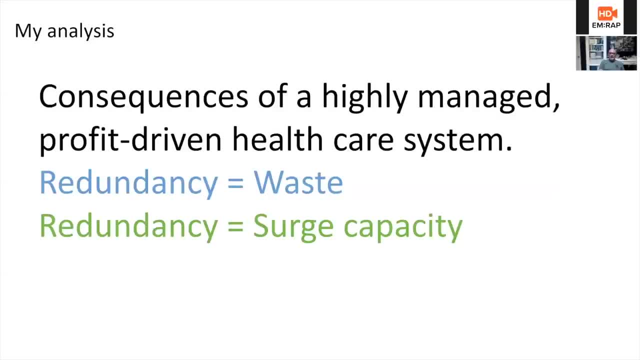 One. it equals surge capacity. If you have empty beds, you have a place to put people who get sick when there are additional people. Others would say redundancy actually is a good thing in society, because hospitals and health care are unique employers in most communities. 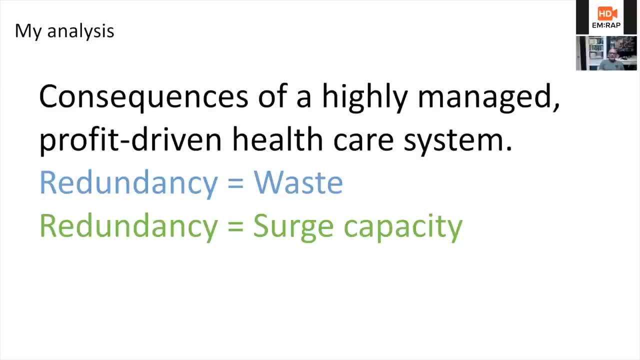 In that almost every community has health care and therefore a source of employment. And secondly, hospitals offer lots of jobs for people who may not be able to compete in the modern high-tech environment: People who work in the kitchen, people who transport patients. 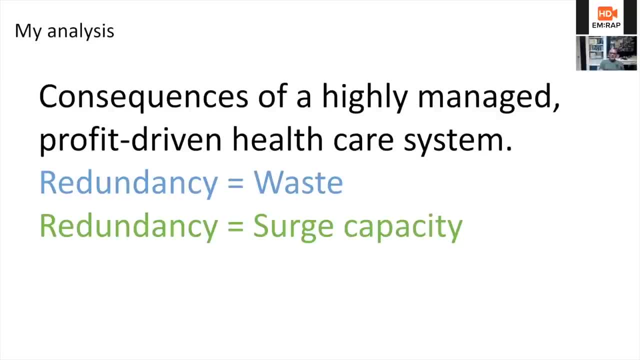 people who clean the place. All of these are jobs which our society needs, and having some redundancy there is not a bad thing for the economics of a community and the well-being of that community, as employed people are. Unemployed people generally fare better. 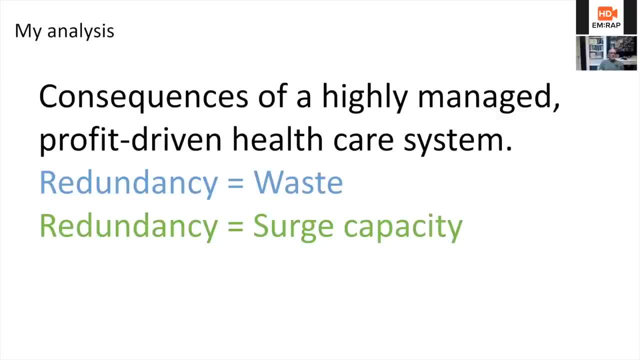 than unemployed people, But in any case two visions of what redundancy means And consequently the capacity and also the distribution of that capacity, meaning where are the beds. Interestingly, in New York City some of the places that most need beds have less beds. 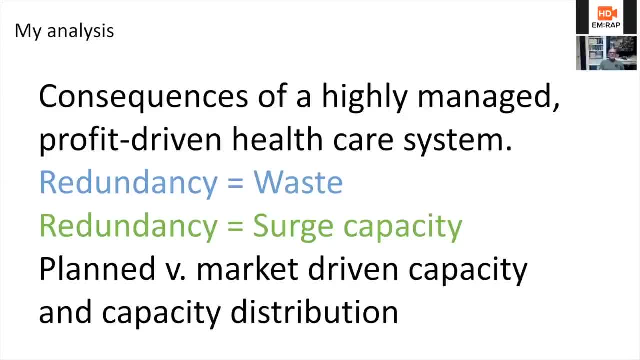 and some of the places that least need beds have more beds. That's a function of the marketplace, putting beds where profit is to be made, as opposed to any type of systematic. But in New York City it's more of a systematic planning. 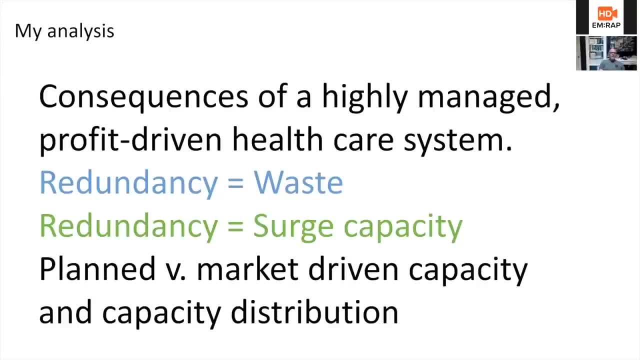 where you place beds and personnel over the long haul, where they're likely to be needed. So, as a consequence of this, we do not have the surge capacity or the appropriate distribution to handle a disease that's worse than the flu, even if it's only mildly worse than the flu. 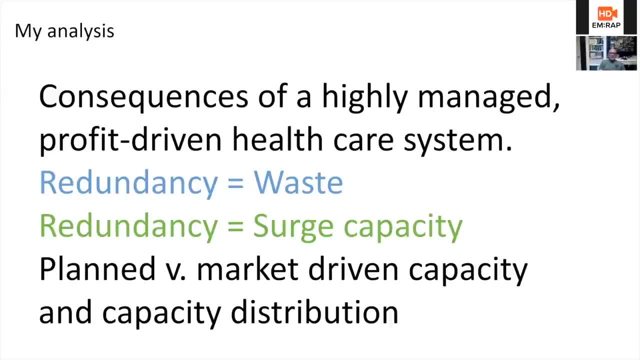 So the argument two people may be right- It's only mildly worse than the flu. But the argument one people are also correct, because our health care system is designed in a way that we can't handle much of a surge at all. So let's look at Sweden. 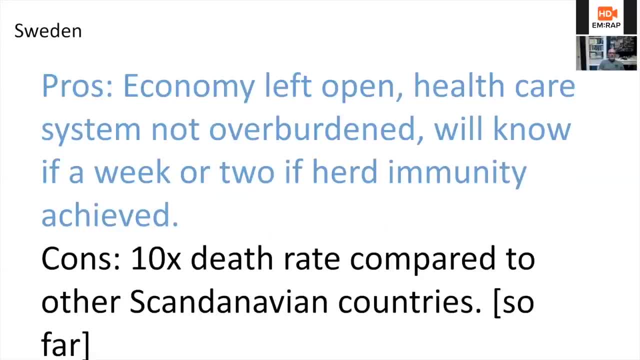 Sweden's one of the few modern countries who've chosen to leave their economy open. They closed graduate education, college, things like that, But they left the schools open. They left most stores open, And yet their health care system is not overburdened. 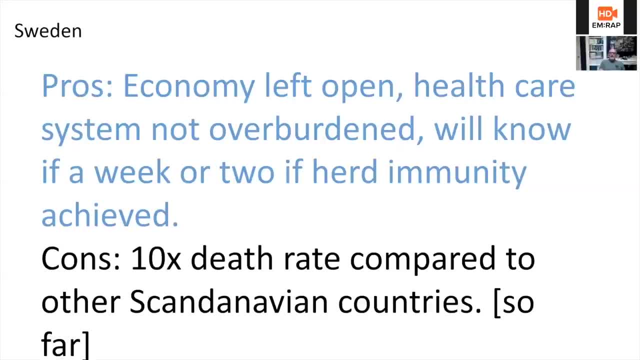 because their health care system is designed to have redundancy And the beds are where they're needed. They're not where the market forces have placed them, And we'll know in a week or two if they really have achieved herd immunity or not. That's the pros. 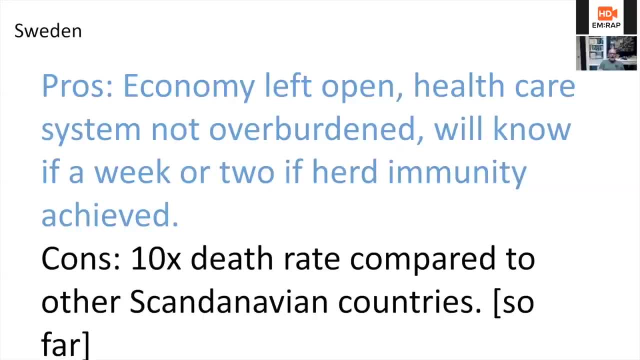 The cons are that their death rate is tenfold higher compared to other Scandinavian countries per capita. That's right now, But if they have in fact achieved herd immunity, so that most of the people who are going to die from this in Sweden have already died, they may just be ahead of the curve. 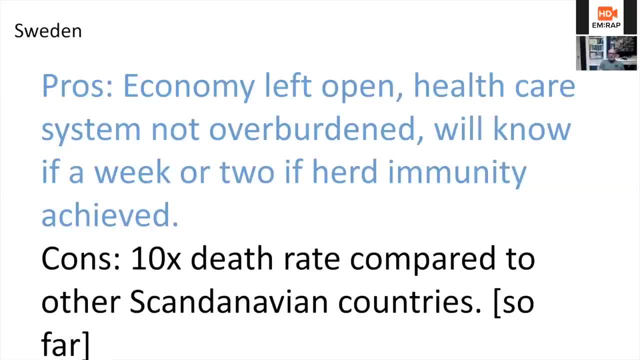 Because in the other countries they have not achieved herd immunity. They only have a couple of percentage of people who are immune And unless a vaccine comes along soon, they will go through additional cycles And they may go through enough cycles to achieve the same death rates that Sweden. 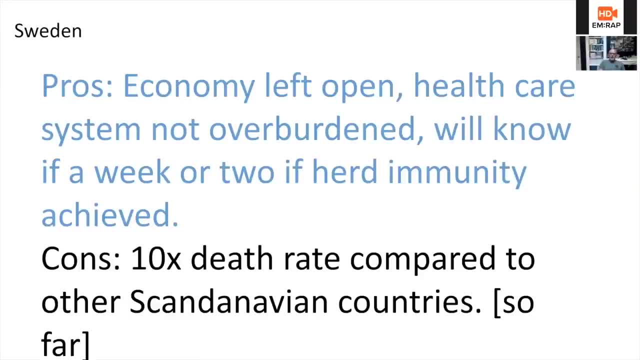 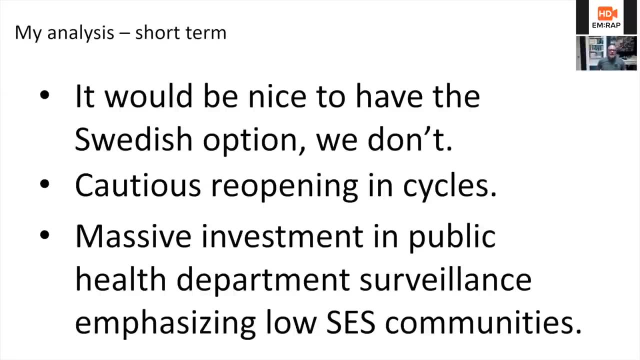 had just over a much longer period of time and with all the negative economic consequences of having been closed for long. So what do we do In the short term? it would be nice to have the Swedish option, but we don't. We simply do not have the human or physical capacity. 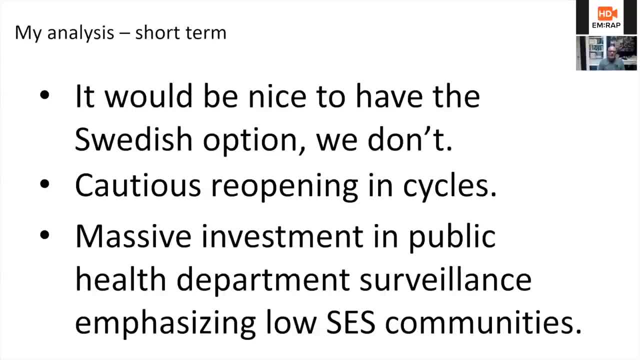 to handle the wave of illness that would occur should we open things up as they are currently. So we're going to have to do this. We're going to have to do this with cautious reopening in cycles and strategic reopening. But even before we do that, we have 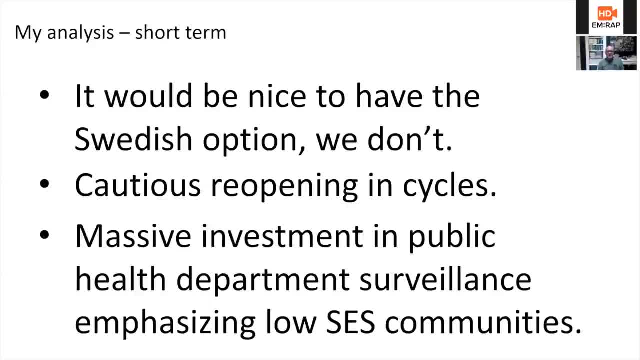 to have a massive investment in the public health department surveillance capacities, emphasizing low SES communities, because they are the most vulnerable and the least capable of isolation. So that's where we really need to have amazing surveillance to detect cases and isolate them and protect others. 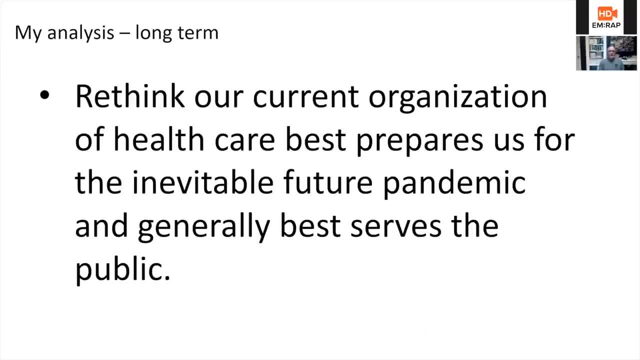 In the long term, I think we really need to rethink our current organization of health care, both the public health aspect of it and the hospital- The public health aspect of it- To find something that better prepares us for the inevitable future pandemics that we'll experience. 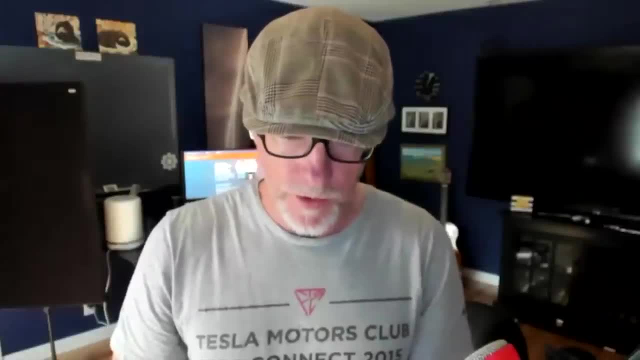 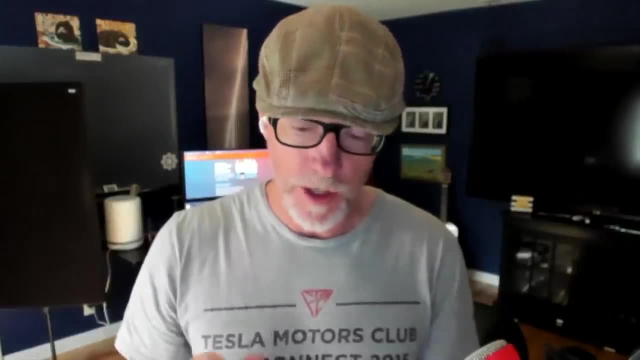 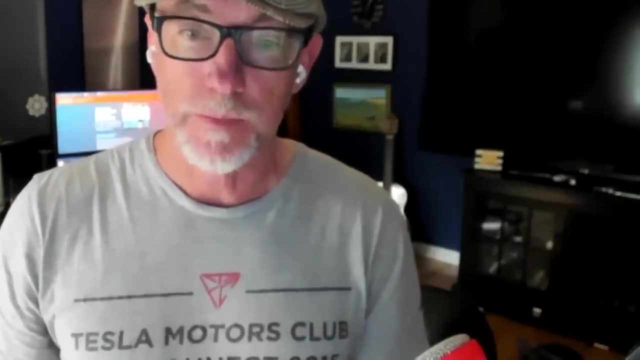 and generally best serve the public. So, Schreiger, tell me what the world looks like if the worst case scenario is there, a worst case scenario where a vaccine doesn't come for a very long time. immunity is not perfect. What does this look like? 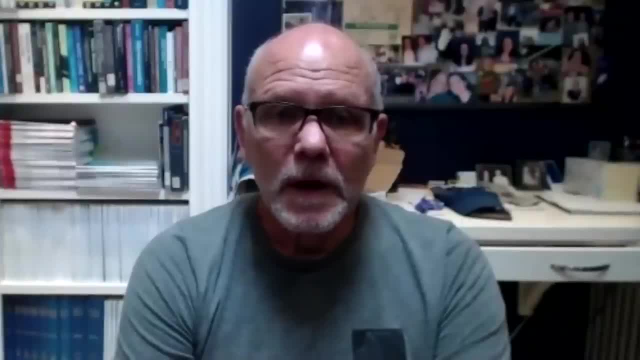 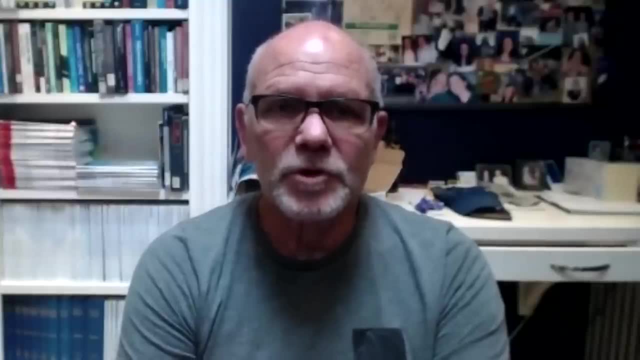 Well, it certainly is concerning Without. incredibly, There are a couple of things you left out, which is: do we have a rapid test which is highly sensitive and relatively specific? If we have that and over the course of time, we develop a sufficient public health effort. 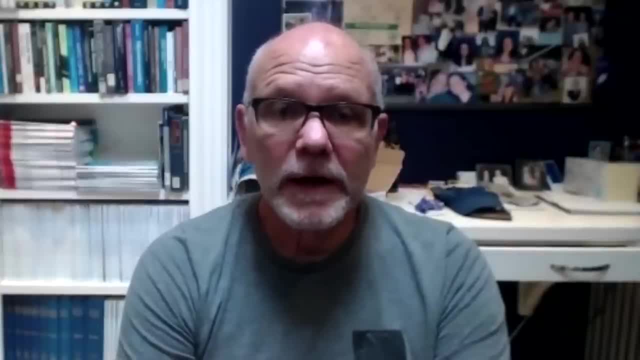 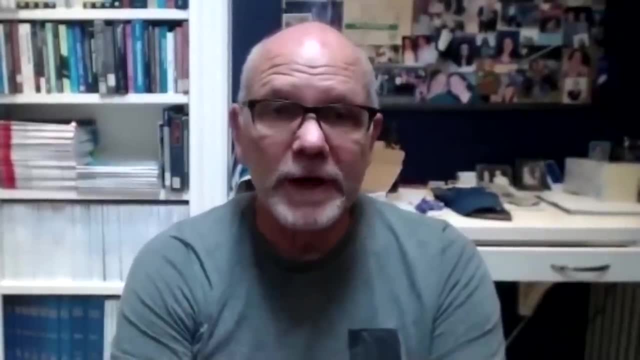 that we could do active surveillance of everyone, track cases, isolate cases and in that way avoid the spread. then there's the potential that we could get control of this. But those are a lot of ifs. We need the test and then we need 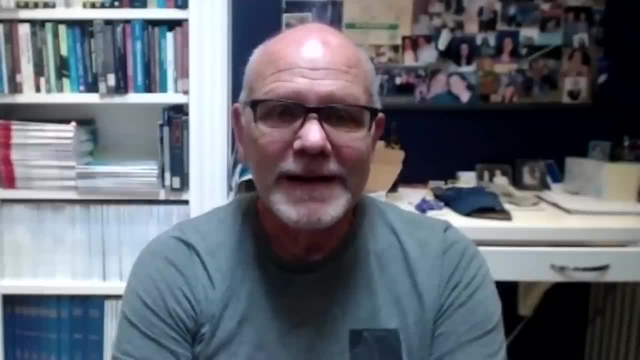 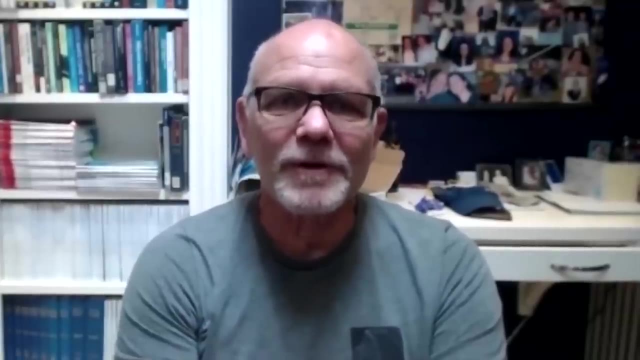 the surveillance. And the question is, is the surveillance going to be sort of 1900s type surveillance where there are a lot of public health workers feet on the ground, chasing, tracing, contacts, interviews, manual labor, talking to people making phone calls? 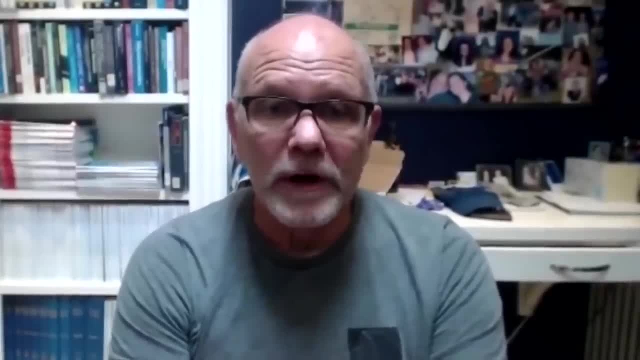 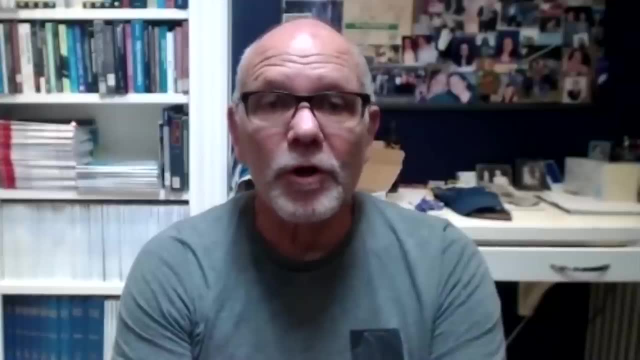 walking the streets finding people, Or is it going to look something like a 21st century kind of techno state with all the groups? Yeah, Yeah, Yeah Yeah. There's good things and bad things about that- where we're doing electronic surveillance. 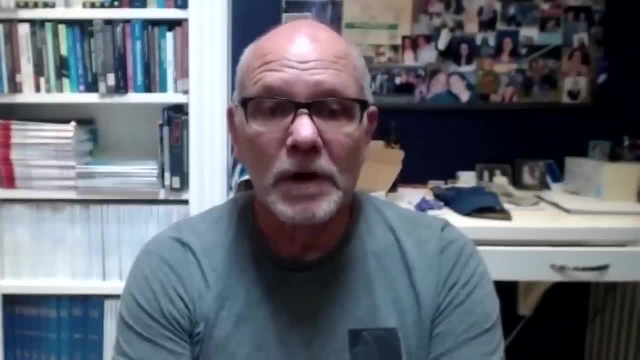 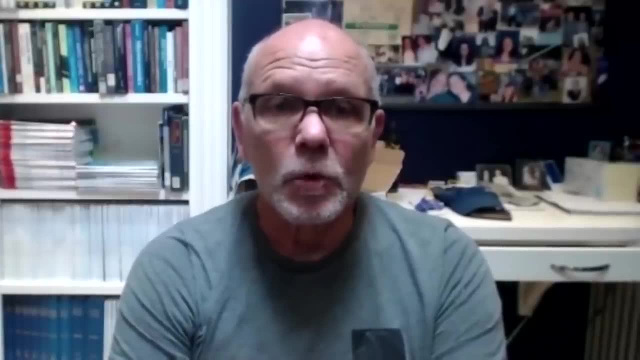 and figuring out electronically who's had contact with whom. Of course, the latter comes with a great potential for removing civil liberties. Would Americans be comfortable getting a phone call saying this is your government? You just were in a store where someone had COVID. 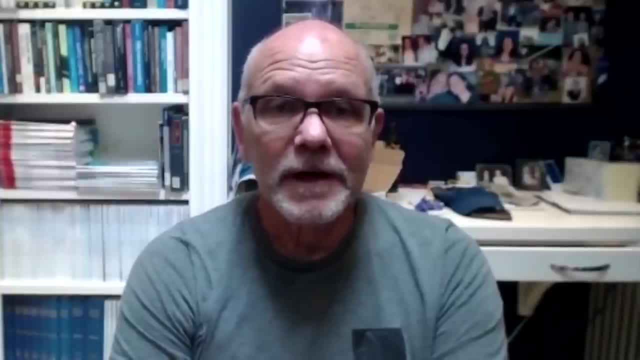 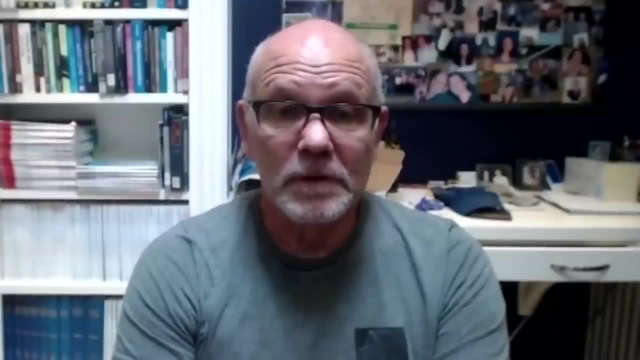 Within 30 minutes of your being there. we need you to isolate, And then they would tell you which store And you would say: how dare you know what store I'm in? Some people would say: thank you, I'm grateful. 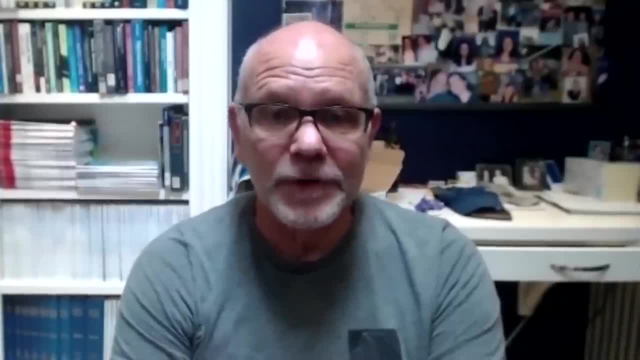 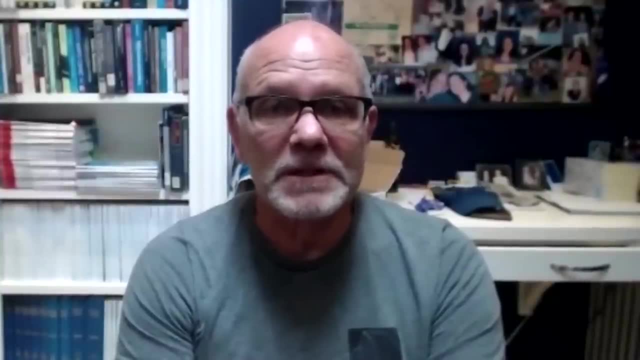 I'm glad that you told me that Others would have a very hard time with it and would also ask the question: well, maybe it's fine in this specific instance, but how do I have any guarantee that this is the only purpose that's being used for? 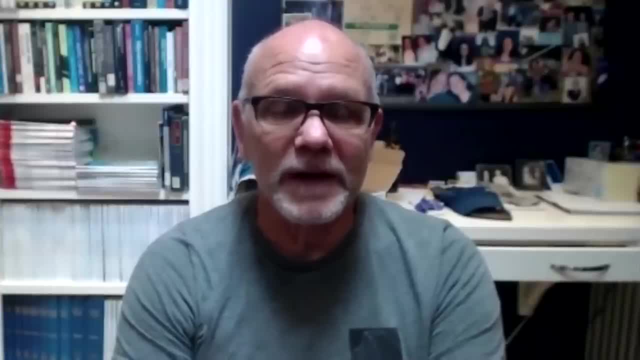 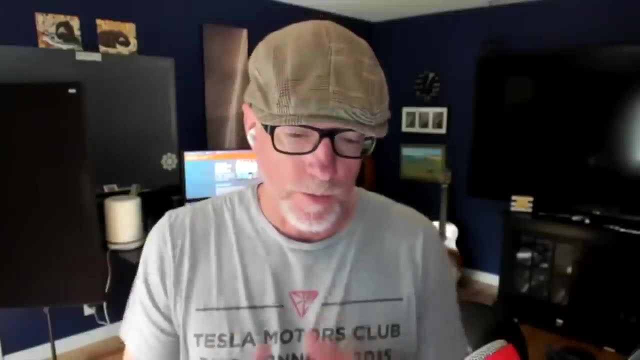 And we're moving into some brave new world police state with surveillance. So we're going to have to wrestle with all those issues if an easy solution doesn't come to this. JOHN MCWHORTER, The other reason to flatten the curve, as you've said, is here in the United States. 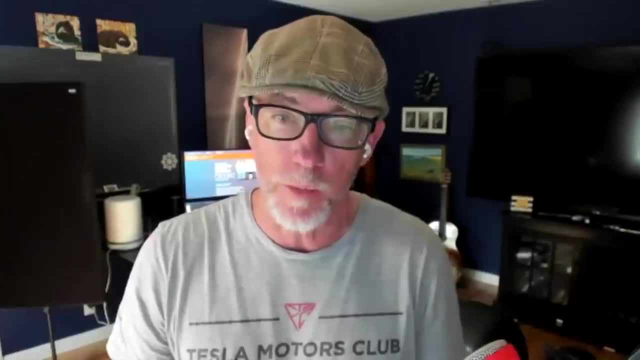 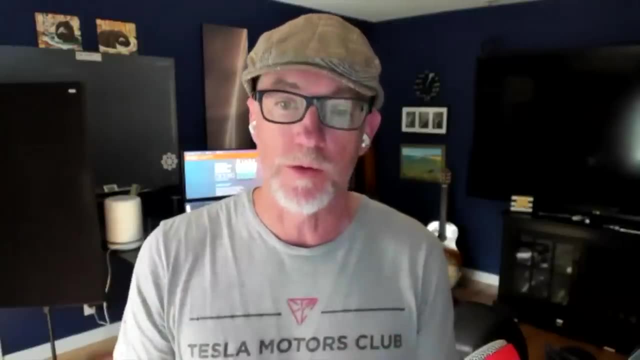 we don't have enough personal protective equipment for our frontline workers. If you just open up your state or the country, you're going to put the people on the front line at an enormous risk. They're going to run out of the stuff that they need. 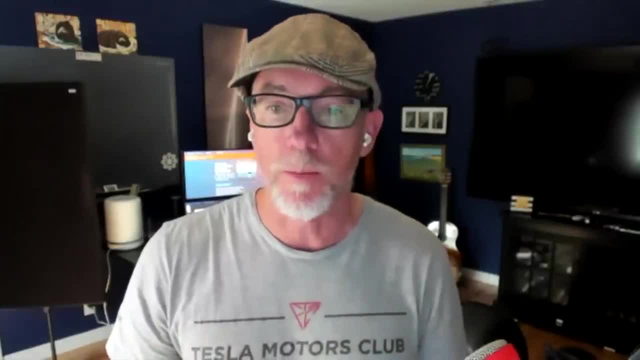 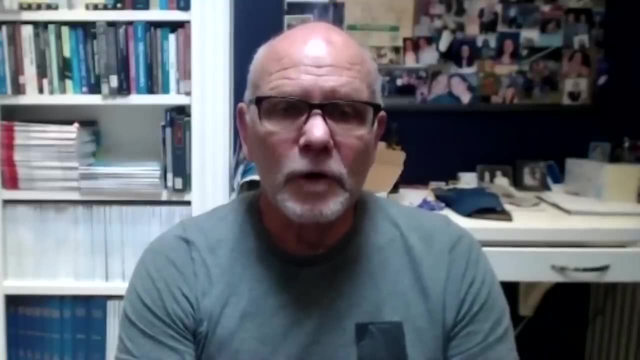 And they're going to have a very high infectivity rate And you're going to kill a whole bunch of them And I would expect that many of them won't come to work. DAVID BASILIS, I think that becomes a really, really interesting question. 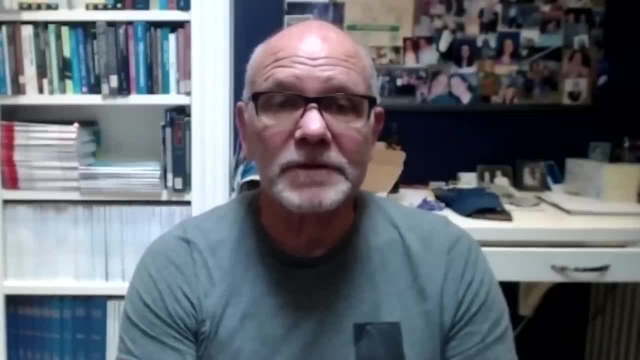 JOHN MCWHORTER, I think that becomes a really really interesting question. DAVID BASILIS, I think that becomes a really, really interesting question. JOHN MCWHORTER, I think that becomes a really really interesting question, Which I mean I've had to deal with myself to some extent. 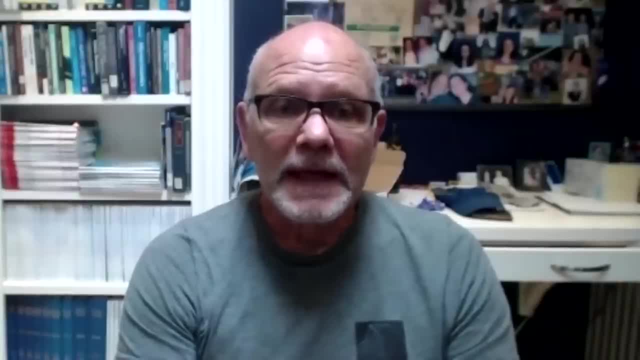 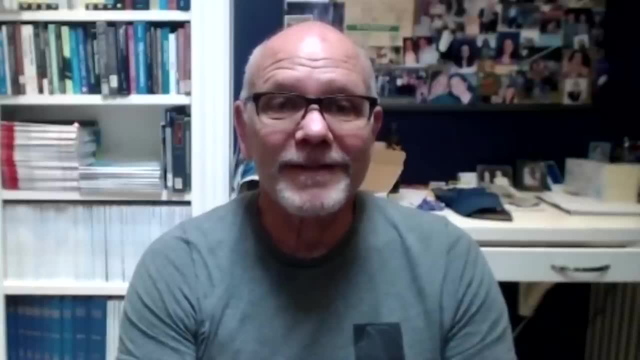 I'm 61 years old And I'm thinking: if things stay this way, if the joy of talking to patients without full PPE on is lost, does the quality of the work at this point warrant my placing myself at risk? Now? fortunately, in LA it hasn't been that bad. 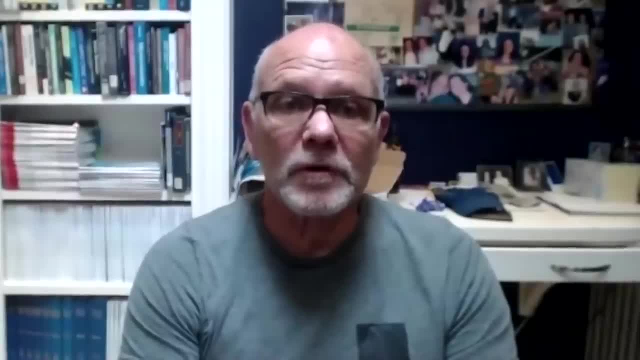 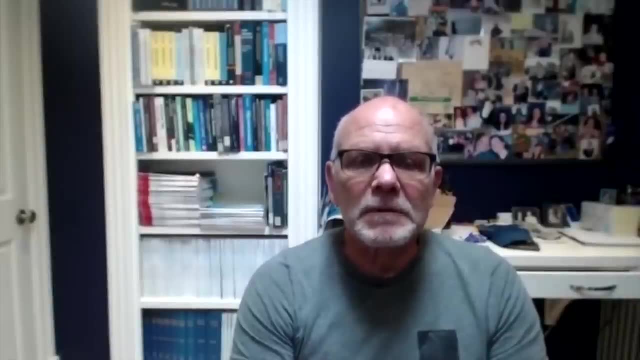 So it hasn't come to that yet, But if we were at the point where it really was like New York, what would I do? I'm still wrestling with that. It was much easier, I think, in previous eras where the physicians felt like this was their obligation. 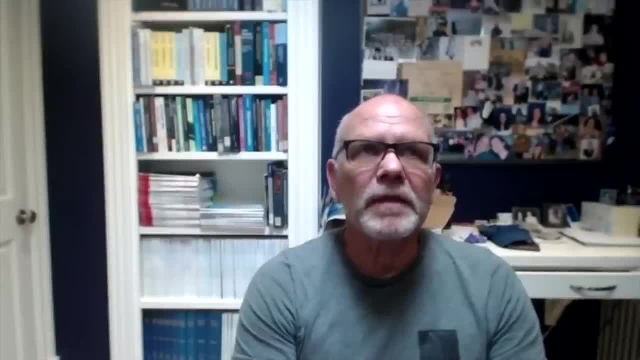 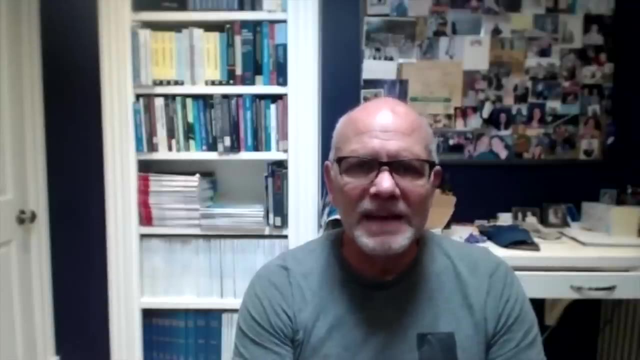 This is what they trained for And they had a moral obligation And they felt good about carrying out that obligation Here, where it's perceived that they're being asked to do things without proper equipment, not because they didn't prepare adequately, but because 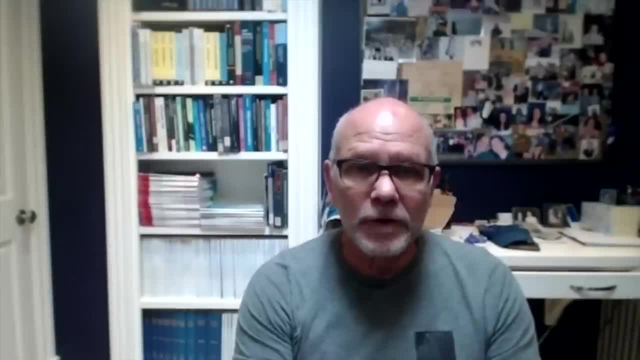 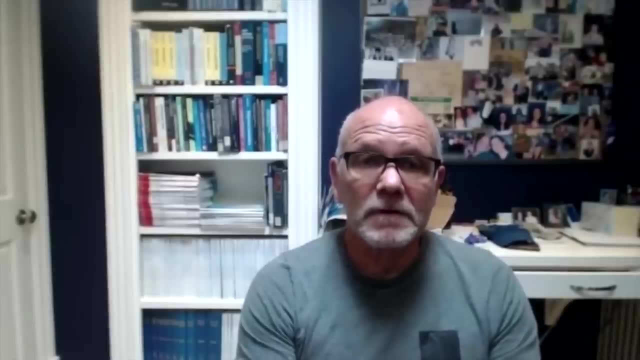 you know the bureaucratic decisions were made, which leaves them vulnerable. it has a different mindset. If I fail to prepare myself, that's a failing of my own, And then I have to live by the consequences of that. But if the failing is due to the government or bureaucracy, 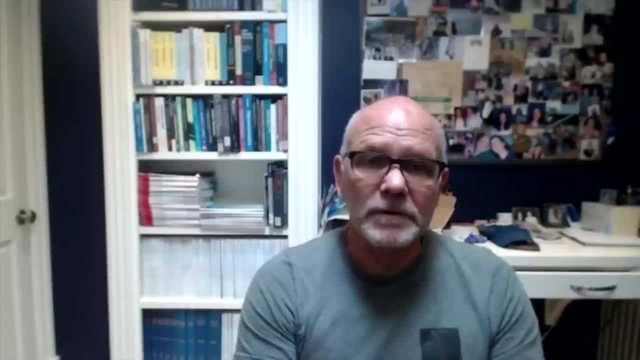 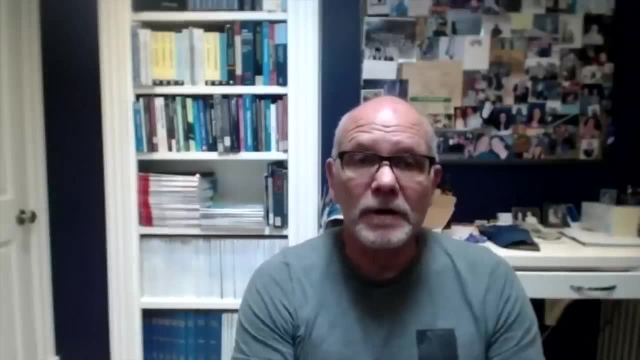 or whatever. what is my obligation in that environment? I don't know the answer to that question, but I'm sure certain people are going to say, well, if you don't give me proper PPE, I'm not going in there. 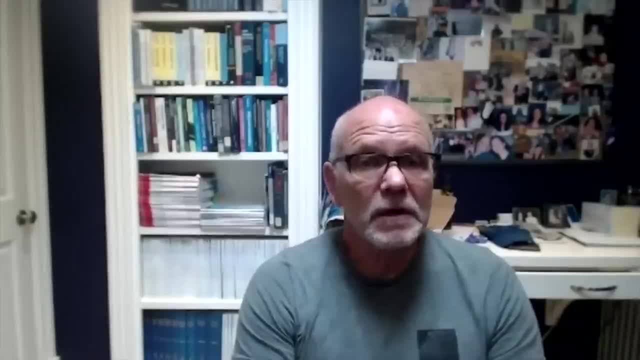 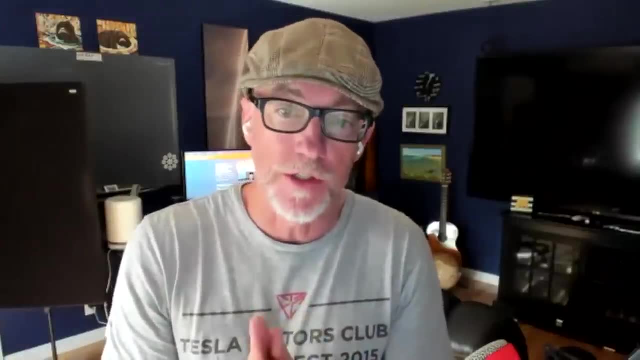 And that doesn't sound like an unreasonable response to me. from one perspective, I don't think it's unreasonable because, unlike walking down the street, there are some procedures that docs and nurses are asked to do that are very high risk, or at least we believe they're very high risk.